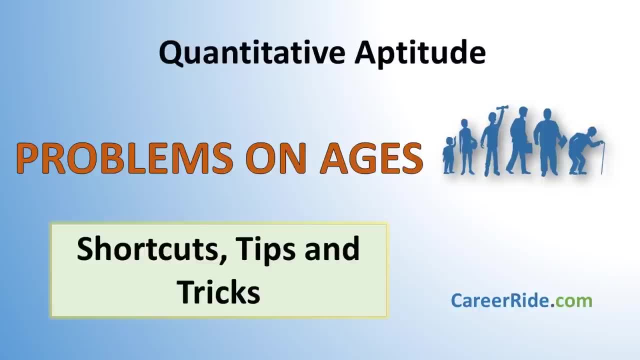 Welcome to quantitative aptitude video on problems on ages from careerrightcom. This is a favorite topic of examiner used to confuse applicants during placement test, job interviews, MBA bank and all other entrance exams. There are always questions from this topic in every exam. This video will give you tips on how to tackle these sums and what to focus on. 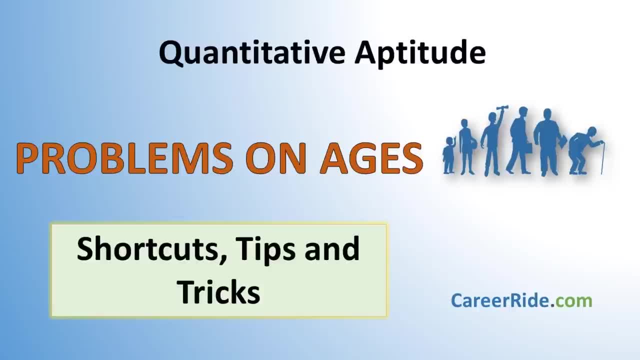 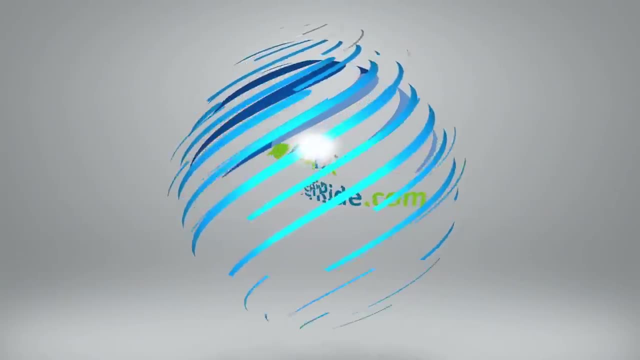 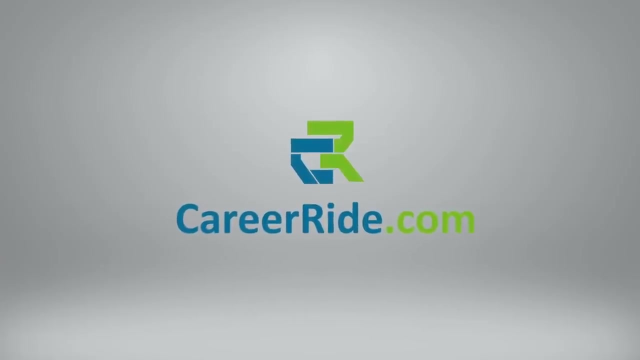 making it faster to solve these easy sums. You can even practice quantitative aptitude on careerrightcom, which has 1000 plus practice questions, and also take the practice test over there. Let's get started. Let's start with an important note. The important note is that 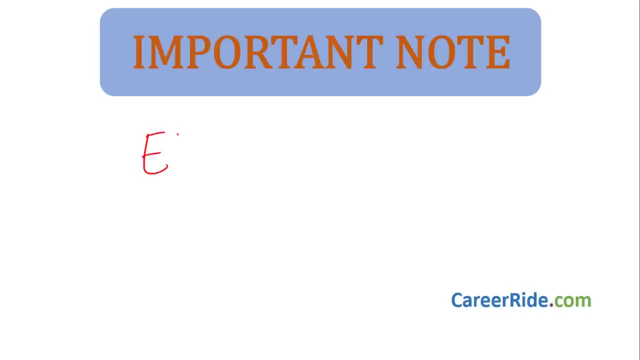 problems on ages are extremely easy. Yes, they are extremely easy. You don't have to remember any formula or anything like that over here. What you just need to remember is that we need to read the question carefully. Once you read the question carefully, once you read the question carefully, you will find. 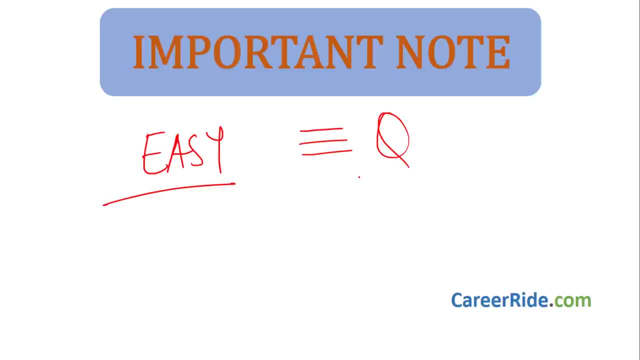 everything in the question. you can construct an equation and solve and get the answer. Okay, so these are very easy. Keep that in mind and you will be able to solve it very quickly. Just pay attention to it. So let's see how to solve questions on ages. 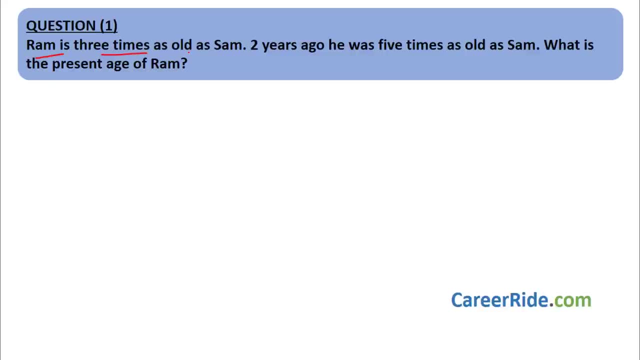 Question number one: Ram is three times as old as Sam. Two years ago he was five times as old as Sam. What is the present age of Ram? See how easy it is. Let's see how to tackle such sums. Let this be present. Okay, the present age of Ram. let it be. 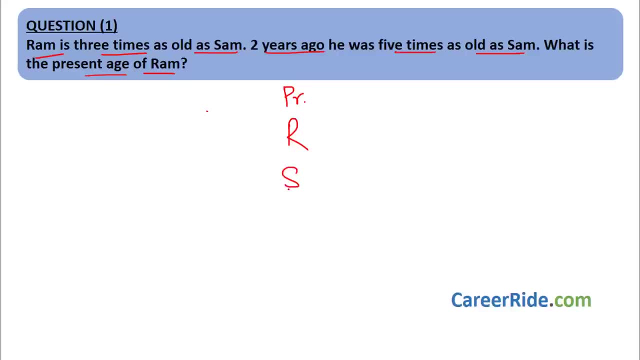 ah, okay, And the present age of Sam. let it be s Now. what they are saying is that Ram is three times as old as Sam. So Ramis three times as old as Sam two years ago. Let's go back. 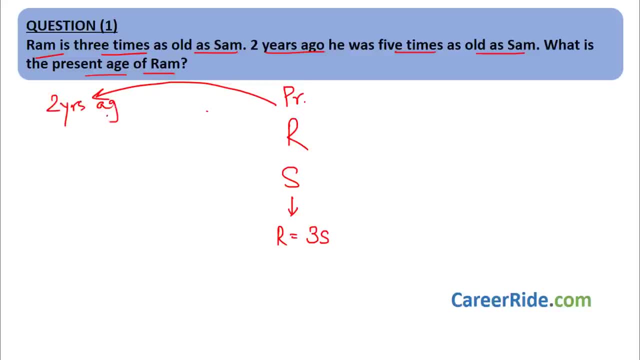 Two years, Two years ago. Right, What will be the age of Ram two years ago? three a –, two, because in two years Ram will grow by two. Ah, Then we can solve this. What is the present age of Sam n2.. 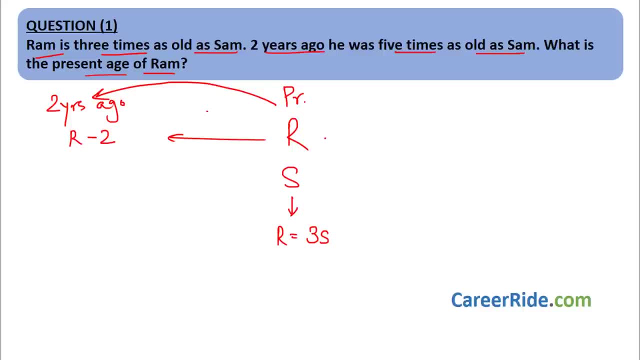 by 2 years. so R-2 plus 2 will be R. that would be present age. so 2 years ago age of Ram would be simply R-2 and age of Sam would be S-2 years. okay, R-2 years, S-2 years, what they have. 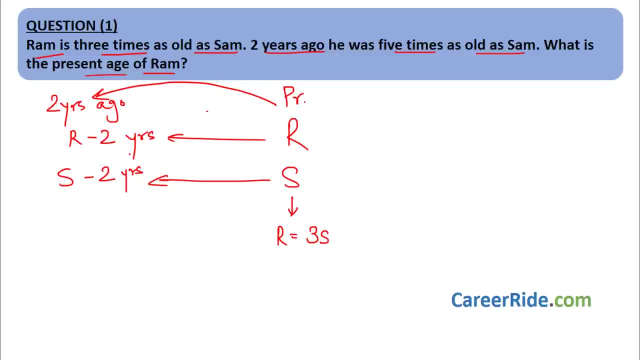 given. 2 years ago, Ram was 5 times as old as Sam. so Ram was 5 times as old as Sam. what is this? R-2 equal to 5s minus 10. okay, now value of R. we know it is 3s. substitute it. 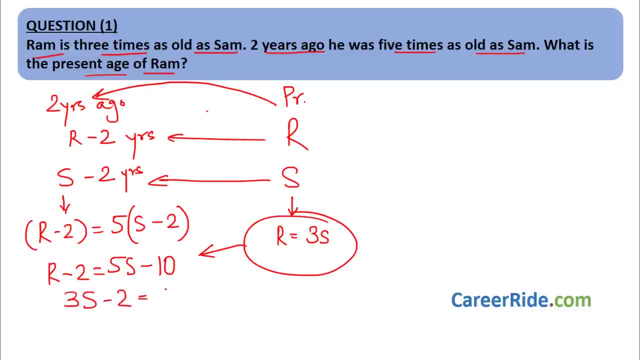 over here. what do we get? 3s minus 2 equal to 5s minus 10. that would be minus 2 plus 10. that would be 8 equal to 2s. therefore, S equal to 4 years. okay, and what do we want? 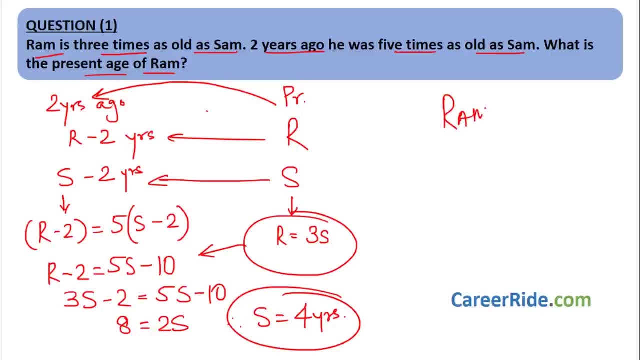 present age of Ram. present age Age of Ram is nothing but 3s, that is, 3, into 4 years, that is nothing but 12 years. okay, so see how easily we got the answer. there is nothing to it if we read the question carefully. 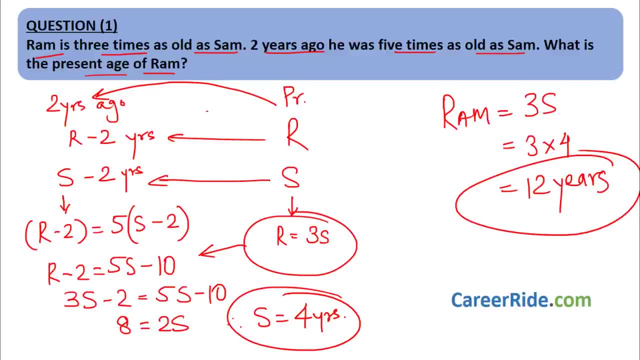 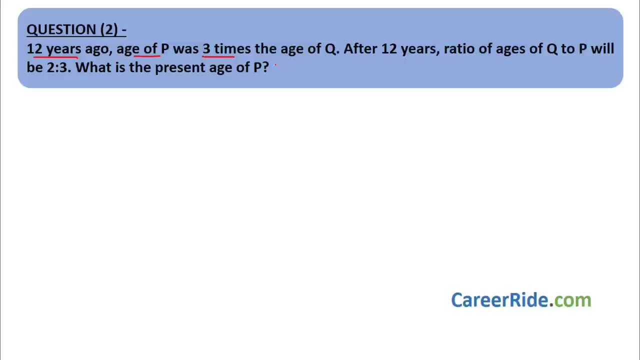 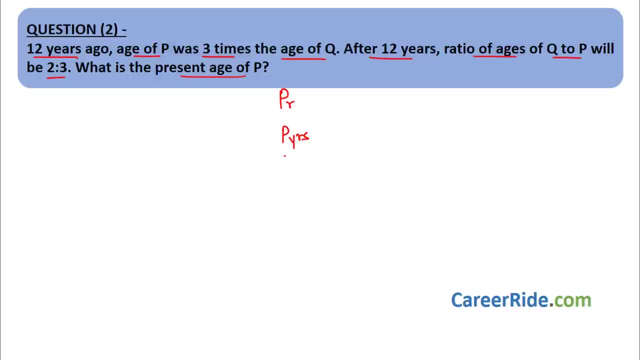 of p, let it be p years, and present age of q, let it be q years. now they say 12 years ago. so let's go back 12 years. so 12 years ago, what would be the age of p? it would be p minus 12 years, right, and 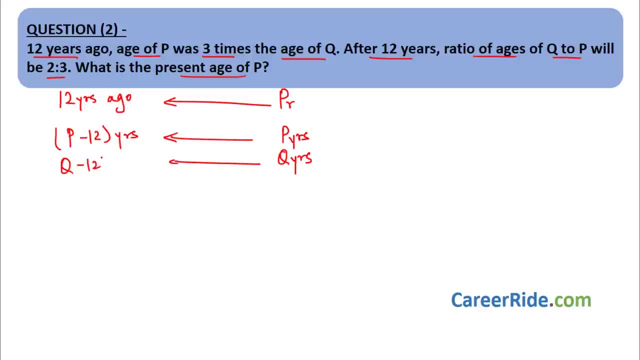 what would be age of q? it would be q minus 12 years. okay, they have given that 12 years ago, age of p was 3 times the age of q. so what we get over here is p minus 12. that was 3 times q minus 12. we. 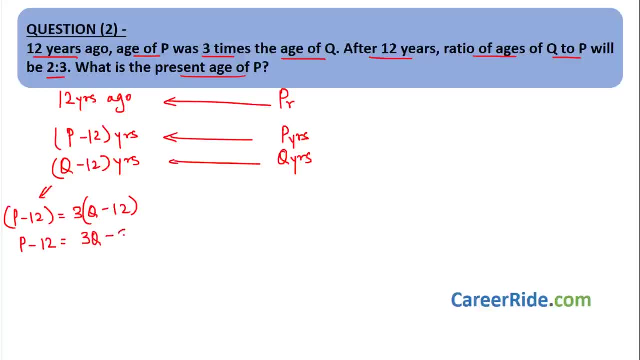 get p minus 12 equal to 3q minus 36. therefore, p equal to 3q minus 24 years. okay, this is the value of p. now what they have given in the second sentence is that after 12 years. so let's go 12 years in the future. 12 years. 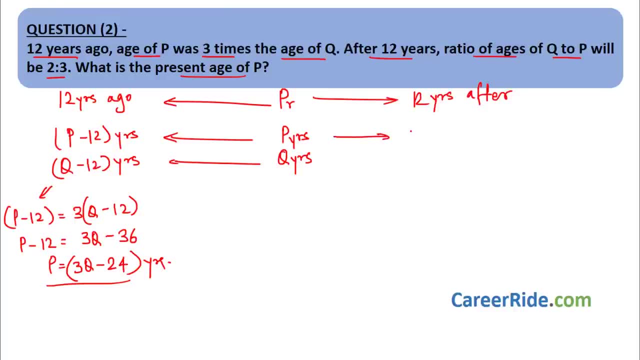 after, okay, 12 years. after. what would be age of p? it would be p plus 12 years. what would be age of q? it would be q plus 12 years, right, p plus 12 and q plus 12. they have given ratio of ages of q. 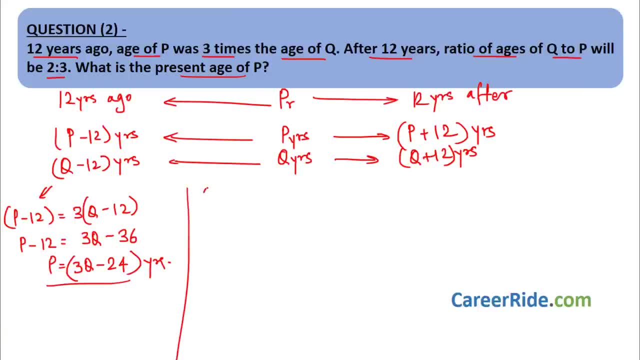 to p will be 2 is to 3. what would be the ratio of age? q plus 12 upon p plus 12? okay, is 2 by 3. now we know the value of p. let's substitute. what do we get? q plus 12 upon. 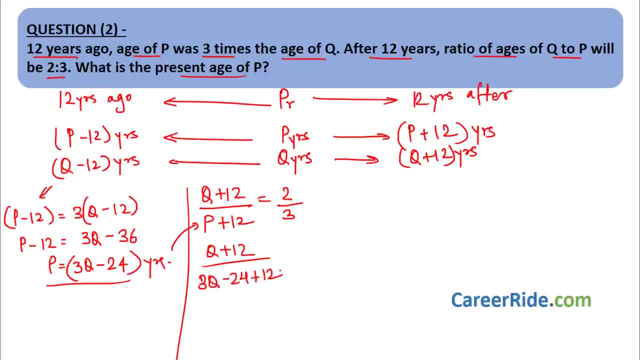 3q minus 24 plus 12 equal to 2 upon 3. we get 3q plus 36 equal to 2, into 3q minus 12, that is 3q plus 36 equal to 6q minus 24. okay, let's solve it over here. what do we get? we get 36 plus 24 as 60 equal to. 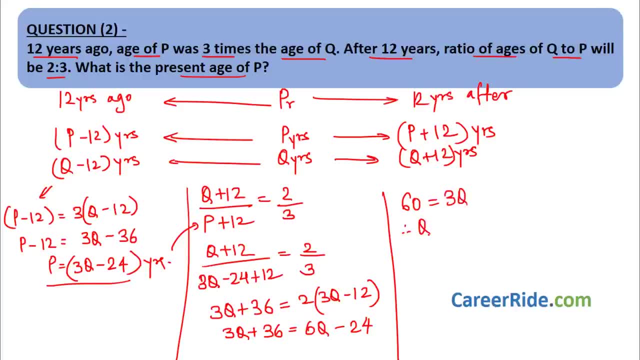 3q minus 3q is 3q and therefore value of q is 20 years. so a present age of q is 20 years. so what is the present age of p? p is nothing but p equal to 3q minus 24. so 3 into 20 is 60 minus 24, that is. 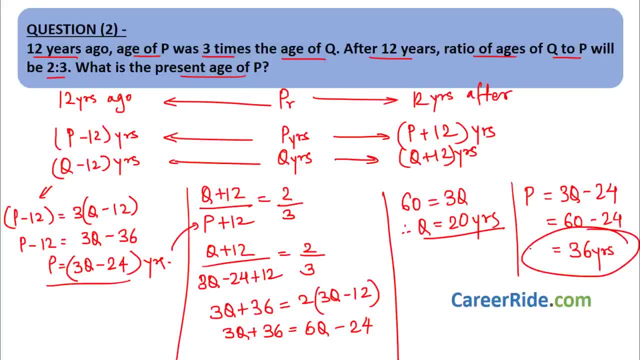 equal to 36 years. so age of p- present age of p- is 36 years. see how we paid attention to this. so we We paid attention to the question, we read the question properly and we were very easily able to find the answer. Moving to question number 3, Rohan is as much younger than Ajay as he is older than Meena. 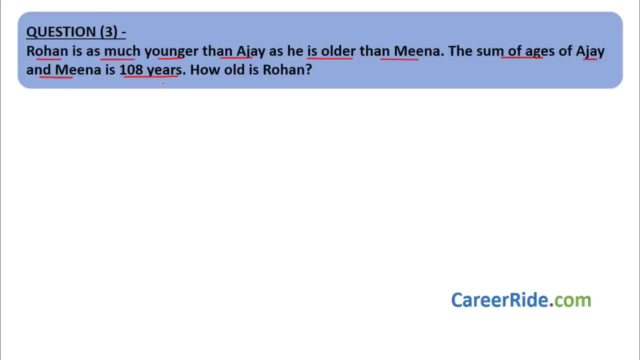 The sum of ages of Ajay and Meena is 108 years. How old is Rohan Now? if you look carefully over here, nothing much is given over here, But if you try to understand the sum, you will find that it is very, very easy. 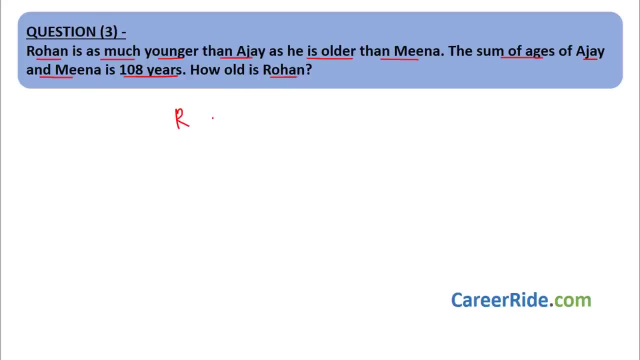 What they say. Rohan is as much younger than Ajay. So Rohan is as much younger than Ajay, So Ajay is older than Rohan. Rohan is younger, or has age less, than Ajay, as he is older than Meena. 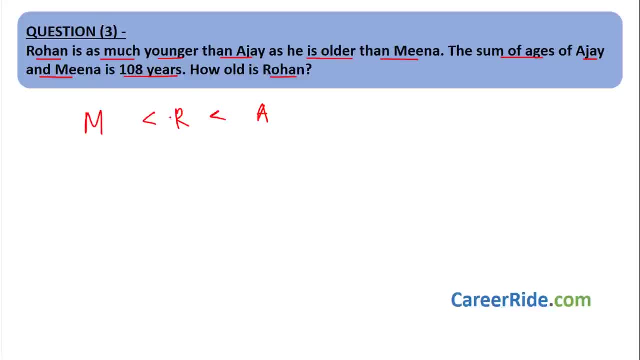 So Rohan is older than Meena and the sentence means that the age difference between Rohan and Ajay is same as the age difference between Rohan and Meena. Okay, Now let us assume another example over here. Let us say there are two numbers, say 10 and 24.. 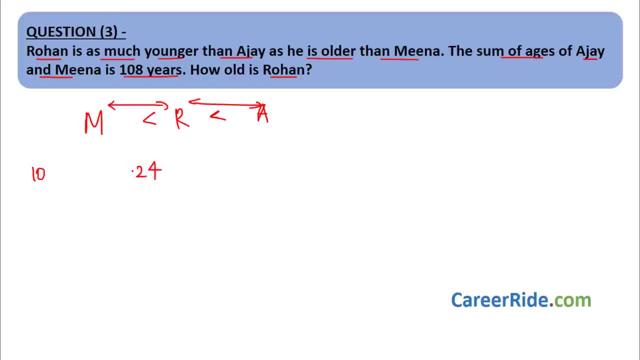 And if someone asks you, between the numbers 10 and 24, which number comes exactly at the center of these two numbers, how will you find out What you will do? you will simply take 10, you will add it to 24 and then divide by 2.. 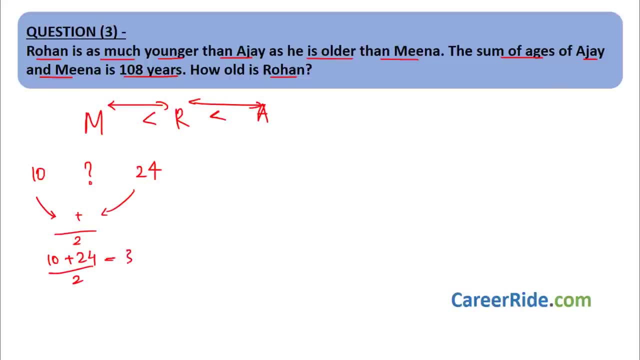 So what? you will get? 10 plus 24 divided by 2.. That is 34 divided by 2. It is 17.. So you will say 17 lies exactly at the center of 10 and 24.. How? Let us see. 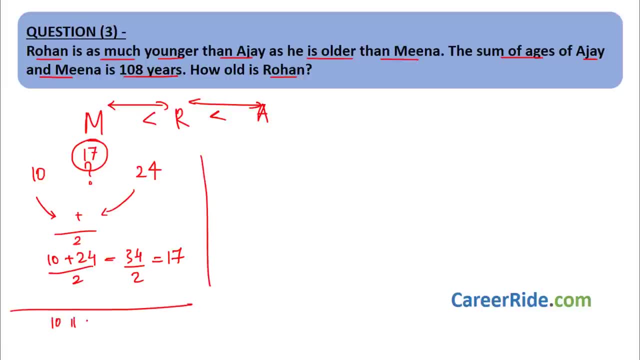 There is this: 10,, 11,, 12,, 13,, 14,, 15,, 16,, 17,, 18,, 19,, 20,, 21,, 22,, 23 and 24.. So, between 10 and 17, what is the difference? 1,, 2,, 3,, 4,, 5,, 6,, 7,, 8,, 9,, 10,, 11,, 12,, 13,, 14,, 15,, 16,, 17,, 18,, 19,, 20,, 21,, 22,, 23 and 24.. So between 10 and 17,. what is the difference? 1,, 2,, 3,, 4,, 5,, 6,, 7,, 8,, 9,, 10,, 12,, 23 and 24.. 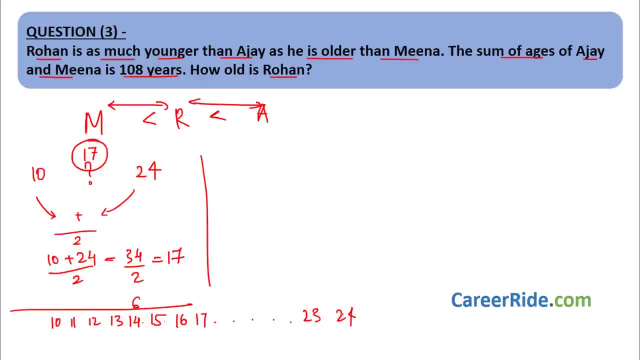 So between 10 and 17,. what is the difference? 1,, 2,, 3,, 4,, 5, 6.. 6 numbers are there between 10 and 17.. Now 17 to 24,. how many numbers are there? 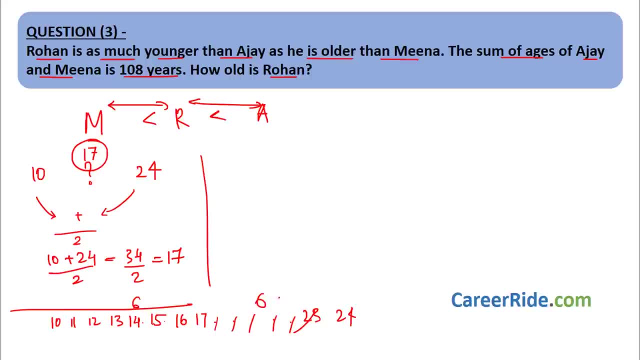 1,, 2,, 3,, 4,, 5,, 6.. See the difference between these two and these two: between 17 and 24, and 10 and 17 is the same 6.. So 17 lies exactly in between 10 and 24.. 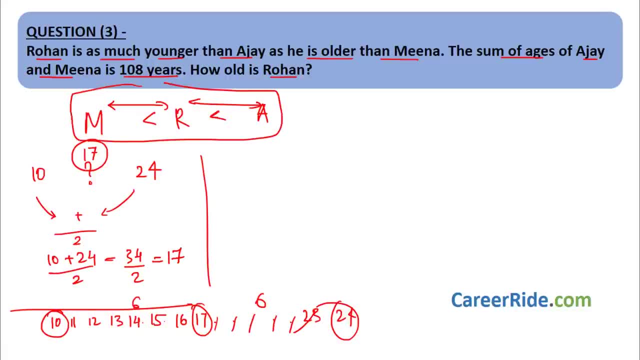 Same way. we have to consider this sum: The difference between Rohan and Ajay's age is same as the difference between Rohan and Mina's age. so what exactly would be the Rohan's age? it would be found out like this: 10 plus. 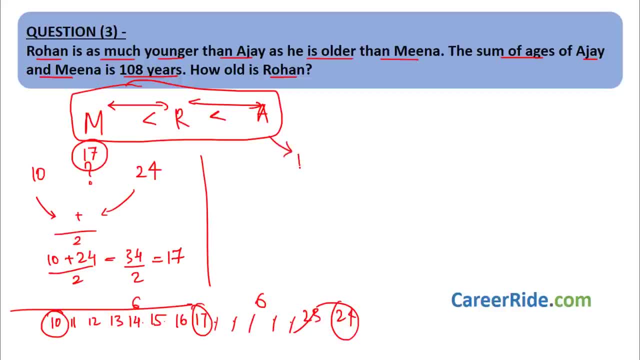 24 divided by 2. same way it would be found out as Mina's age plus Ajay's age divided by 2. but we already know that sum of ages of Ajay and Mina is 108. so we will have 108 divided by 2, equal to 54 years. so, Rohan, how old is? Rohan is 54 years old. see how easy. 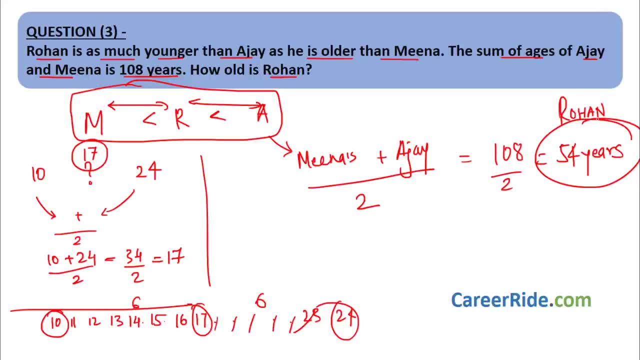 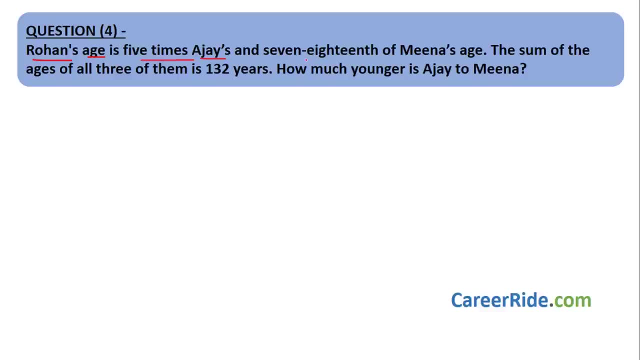 it was with common sense we were able to solve this sum. moving on question number 4, Rohan's age is 5 times Ajay's and 7 18th of Mina's age. the sum of the ages of all three of them is 132 years. 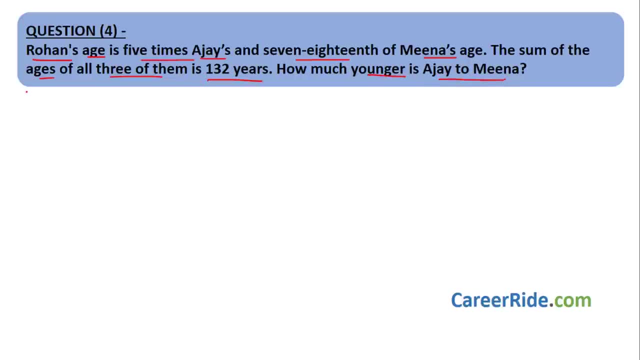 How much younger. What is Ajay to Mina? again, an easy sum. let us assume that Ajay's age be a years. okay, Ajay's age be a years. so what would be Rohan's age? it would be 5, a years right now. Rohan's. 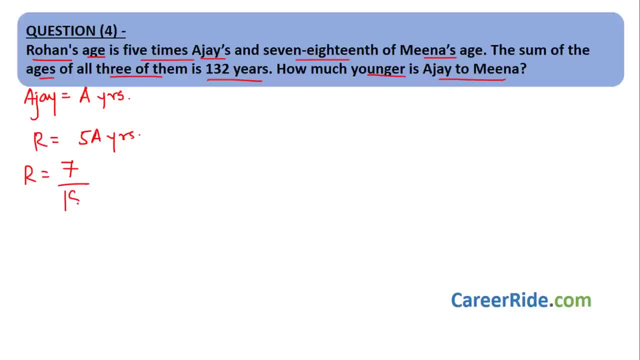 age is also 7 by 18th time of Mina's age, right? so what is Mina's age? Mina's age is nothing but 18 by 7 times of Rohan's age. So what is Mina's age? It is Rohan's age, but we already know Rohan's age as 5 a years. 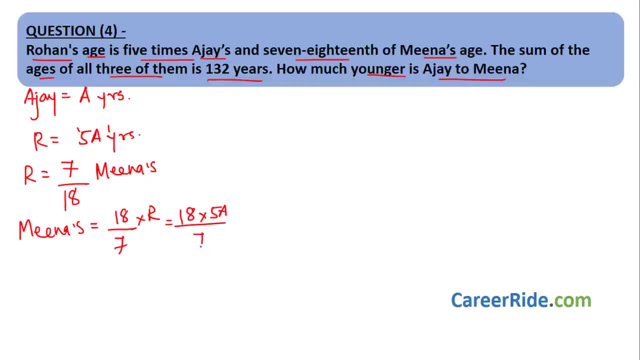 So that would be 18 into 5 a divided by 7. that would give us 90 a by 7 years. Now they have given the sum of ages of all: 3, that is Ajay's age, that is a years, plus Rohan's age, that is 5 a years, plus Mina's age, that is 90 a upon 7 is nothing but 132. 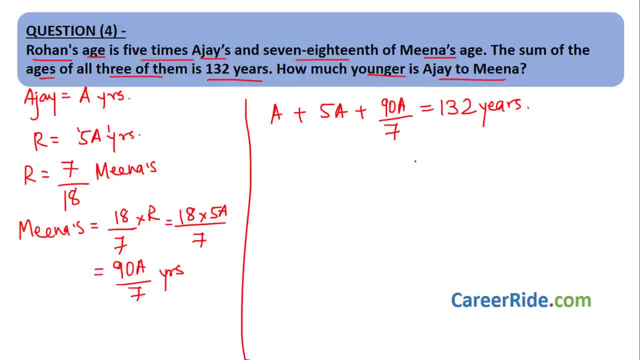 years, right? So we have given 7 years. So what is Mina's age? So how much younger is Ajay to Meena? Let's find out. We have here 6a plus 90a by 7, equal to 132.. Let's multiply by 7 throughout, You get 42a plus 90a, equal to 132 into 7.. Here you get 132a, equal to 132, into 7.. 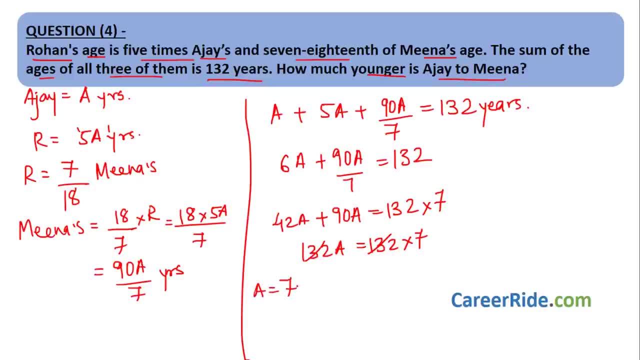 132 gets cancelled. That is, Ajay's age is 7 years. Therefore Rohan's age is 5 times a. 5 times 7 is 35. So 35 years. And Meena's age is nothing but 90 into a upon 7.. That is 90 into 7. divided by 7 is nothing but 90 years. 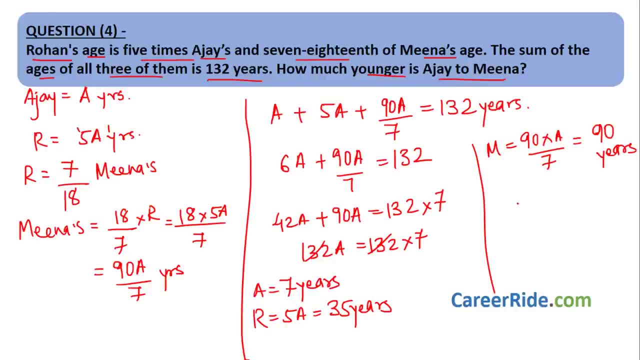 So how much younger is Ajay to Meena? 90 years minus a 7 years, That would be 90 minus a 83 years. So Ajay is 83 years younger to Meena. Right Going to next question. 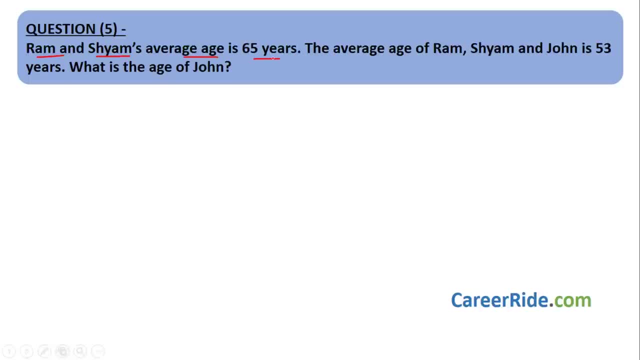 Question number 5.. Ram and Shyam's average age is 65 years. The average age of Ram, Shyam and John is 53 years. What is the age of John Now over here? it is not just problems related to ages. A different type of problem related to ages. 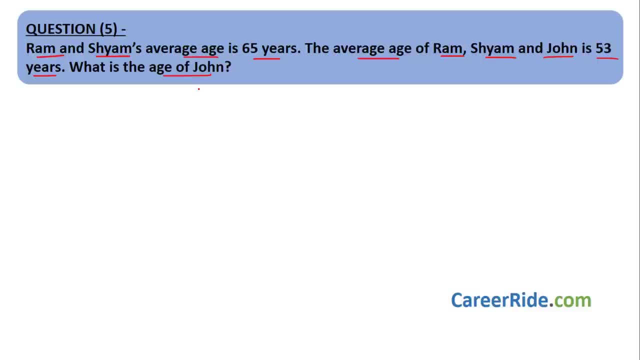 Has been asked over here. It is related to average age. There is not much difference actually. I will just explain to you the small concept related to averages. You can check out the averages video which has been published, So that you will be able to understand what exactly is going on over here. 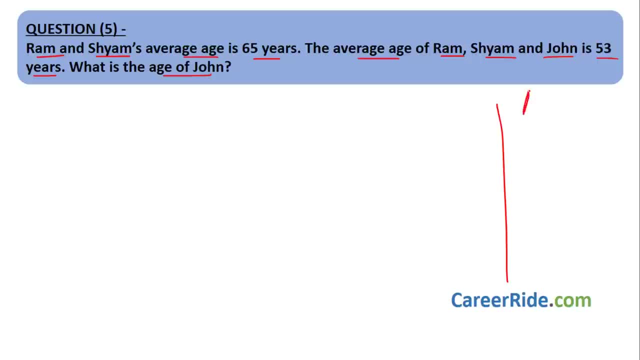 So averages is pretty easy. There is nothing much On the right hand side. I will explain what exactly average is. Now. average means equitable distribution. That means if you have 100 rupees and you have to distribute, Distribute it among 5 children. What you will do is you will just give 20-20 rupees to each of the 5 children, So every person gets same amount of money. That is 20 rupees. 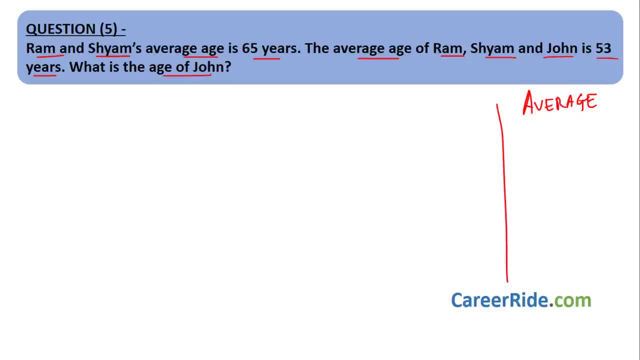 So 20 will be the average amount of money received by each child. That is nothing but average. How to find average? Very easy: Average is sum of all the observations divided by total number of observations. What does that mean? For example, here there are 2 people, Ram and Shyam. 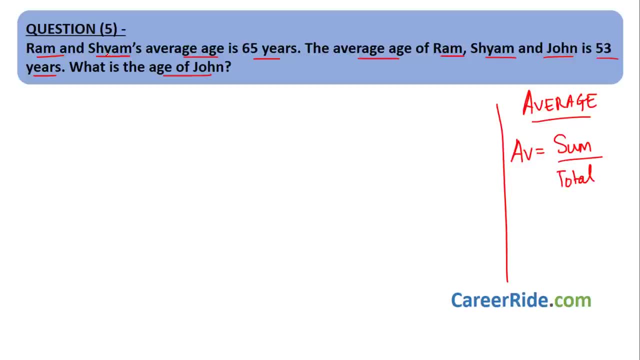 Okay, So there are 2 people, So there are 2 observations, So number of people or total number of observations is 2 over here And age of Ram is say 5 years And age of Shyam is say 15 years. 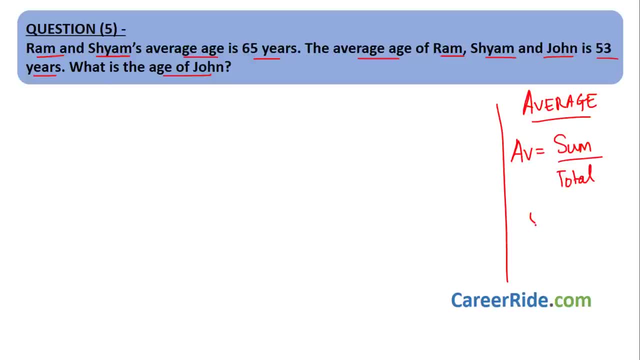 So when we add that, 5 plus 15, what we will get, What we will get over here, 5 plus 15, we will get as 20.. Right, So we will get 20 over here. So this is nothing but the sum. 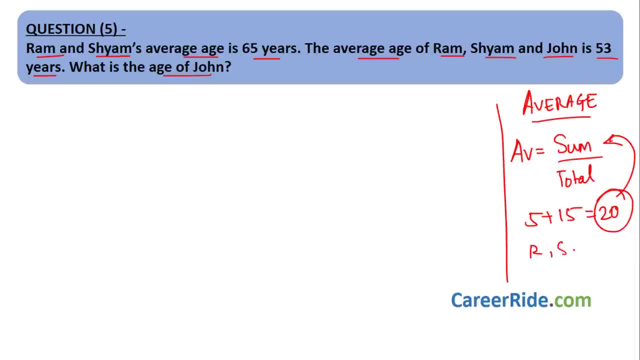 And total number of people are 2.. Ram and Shyam: Only 2 people are there, So total is 2.. Right, So this is total. We just divide this and we get the average. Okay, Let us use this concept to solve our sum. 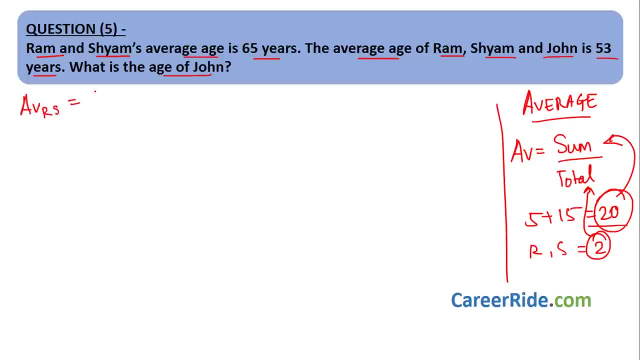 Now, average age of Ram and Shyam is given as 65 years. Okay, Average age of Ram and Shyam is given as 65 years, But we know what is average. That is nothing but sum of the ages, of sum of ages of Ram and Shyam. Okay, Ram and Shyam divided by total number of people. 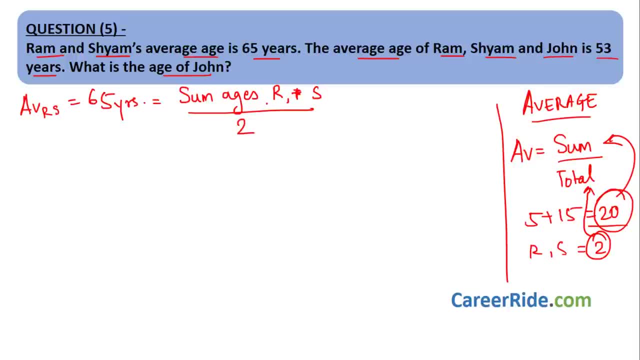 are there just ram and sham- two people, so that would be two. now, do we know age of ram? no. do we know age of sham? no, let us assume that age of ram is r, age of sham is s. okay. and there's a third person over here, john. let us assume john's age be j. okay, now, 65 is nothing but age or sum of ages. 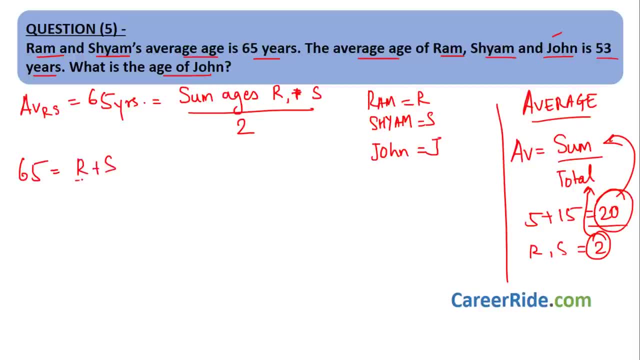 of r, ram and sham. so r plus s, r plus s, is equal to 2, so r plus s would be 65 to the 130 years. okay, now let's come to another scenario. what they've given average age of ram sham and john is 53 years. so average age of ram sham and john is 53 years. that, in that, is nothing but age of. 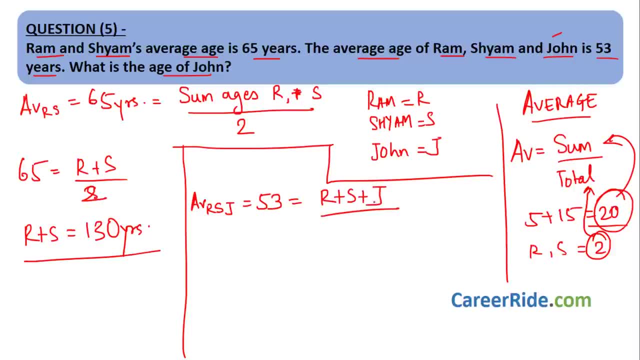 ram plus age of sham plus age of john, divided by total number of observations, how many people are there? right now? there are ram sham, john, that is three people. so divide by three. so r plus s plus j, equal to 53 into 3. okay, 53 into 3 that comes out to be 159. 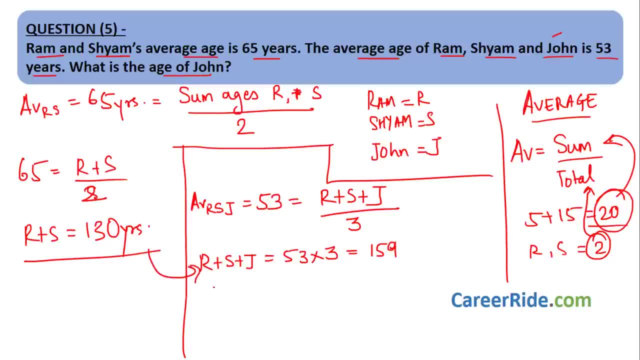 do we know r plus s yes from over here. put it. put the value over here, you will get j equal to 159 minus 130. that would be 29 years. so age of john is nothing, but you could do something like this. you could do something like this. you could do something like: 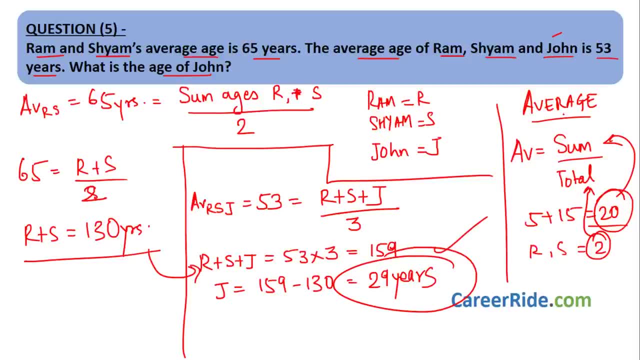 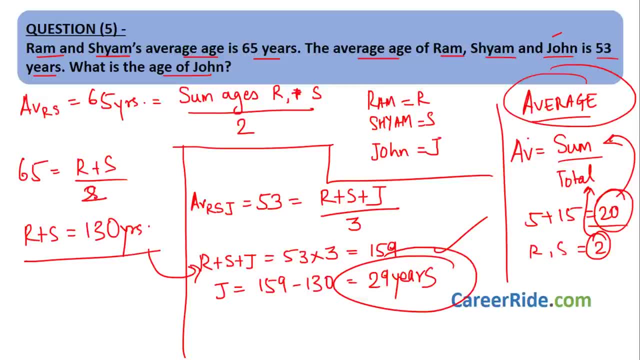 secondary thing. I have explained it in very short. Just remember: average is nothing but sum upon total. But next few questions which are there. they are related to averages and we will be dealing with this in detail over there too, But it is advisable to check out the averages. 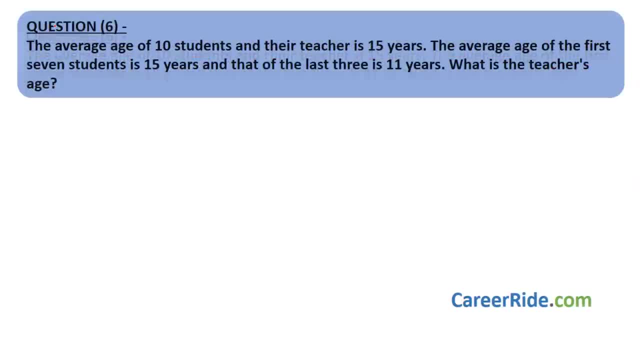 video. Moving to the next question, Question number 6.. The average age of 10 students and the teacher is 15 years. The average age of first 7 students is 15 years and that of the last 3 is 11 years. What is the teacher's age? Again, here we have the average age problem. So what is the? 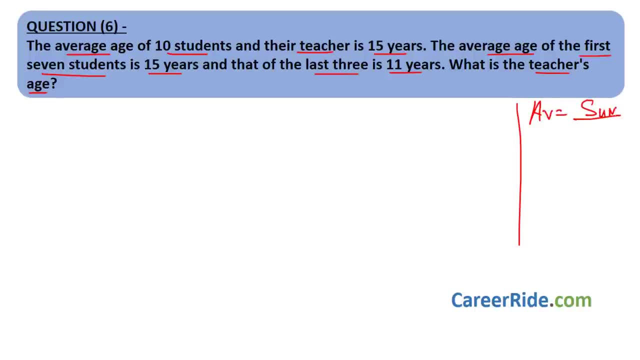 formula for average We know: sum of all observations divided by total number of observations. So in this case what we will have, Average, is equal to sum of the ages of all students, or all people. So people means students plus teacher divided by total number. 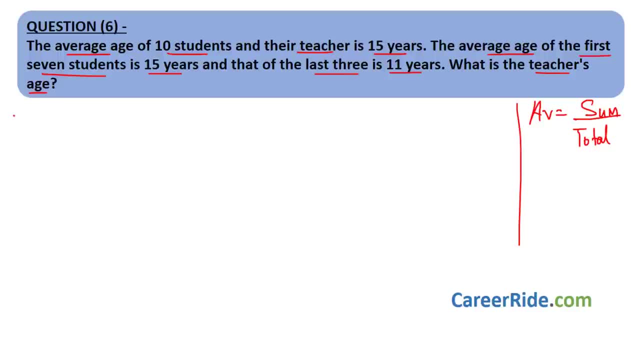 of people, that is, the students plus teacher. So what we will have over here- in first sentence they have given average age of 10 students plus their teacher- is 15 years. And what is average? Average is nothing but sum of ages of all the people. that is sum of the ages. 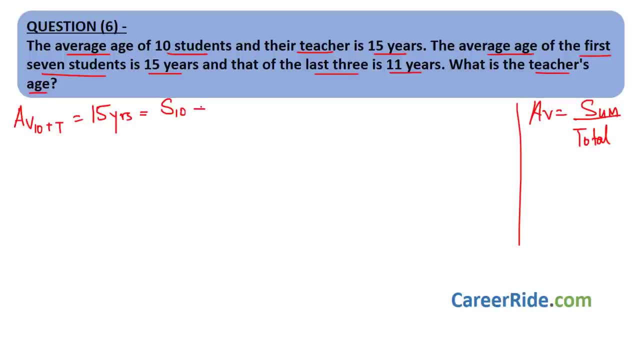 of the 10 students, Let that be S10, plus the age of teacher, Let that be T. So let the age of teacher be T divided by total number of people, that is, 10 students plus one teacher would be 11.. So sum of: 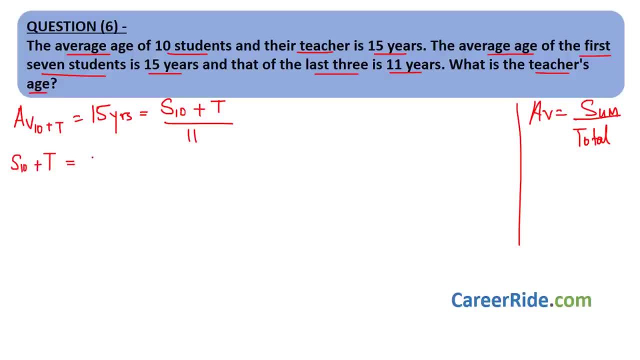 the ages of 10 students plus the age of teacher would be 11 into 15. that is 165 years. Now what they have given average age of the first 7 students is 15 years. Now we know there are 10 students. 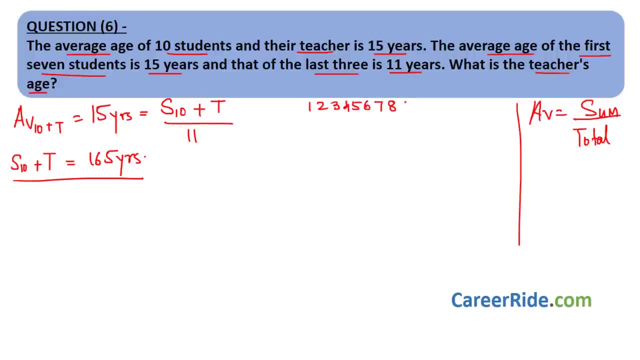 1,, 2,, 3,, 4,, 5,, 6,, 7,, 8,, 9 and 10.. So out of that, they have given that some average age of the first 7 students is 15 and the last 3 it is 11.. So what we will write: average age of the first. 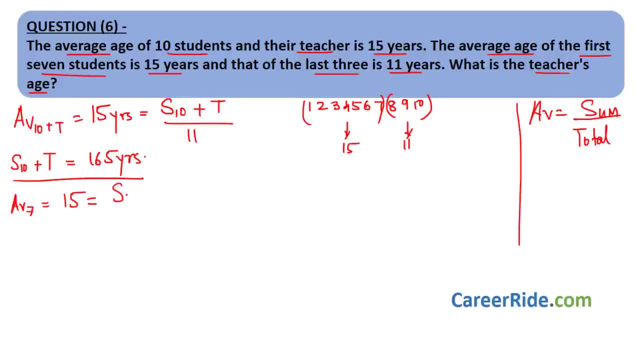 7 students is 15 years. that is nothing but sum of the ages of the 7 students divided by total number of students. Here average we are taking of 7 students. So the total number of people or total number of students would be 7.. So sum of the ages of 7 students. 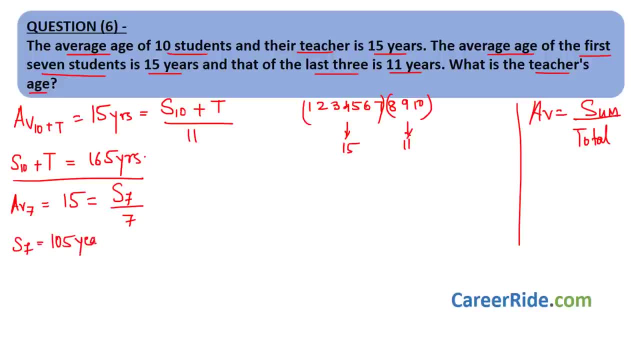 will be 15 into 7 as 105 years. Okay, Same way. average age of last 3 students is 11 years, Right? That would be equal to sum of the ages of 3 students divided by total number of students. that is 3.. So S3, that is, sum of the ages of 3 students, is 33 years, Right? This is okay. This. 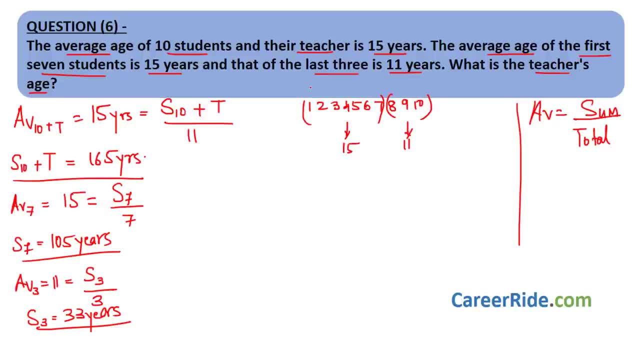 is clear. Now look over here. If we want the summation of ages of 10 students, Okay, What we will do. we will add individual ages. this plus this plus this is, this is, this is, or what we can do. we can add these 7 ages. Then we can again add it into these. 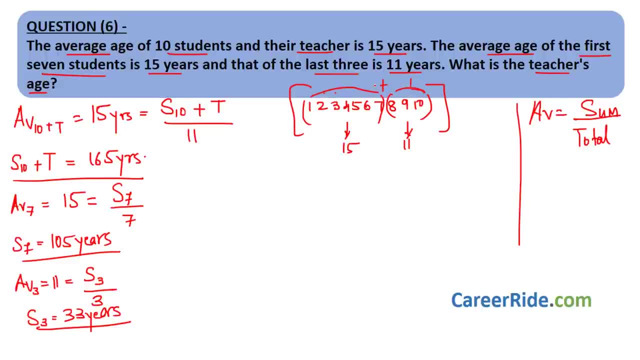 last 3 ages, Right. So we can take summation of this and add it. with this summation, that is the sum of the ages of 7 students. So summation sum of ages of 10 students is nothing but sum of the ages of first 7 students plus sum of the ages of last 3 students. Why? Because 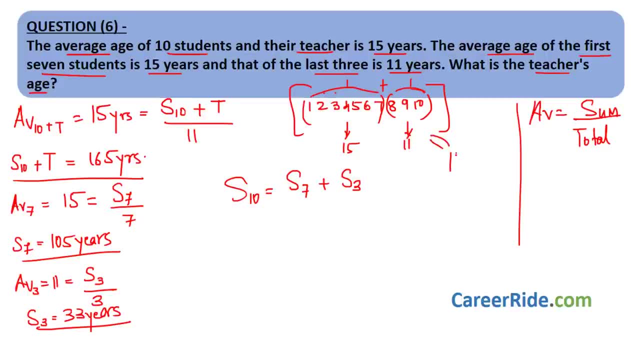 first, 7 and last 3 together make 10 students in total. There is no overlap or there is no one left out? Okay, In total, 10 students can be divided as first, 7 and last 3.. Correct, So same way. 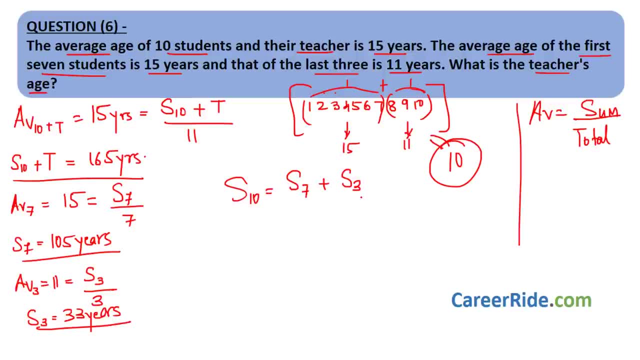 Sum of the 10 students is sum of the ages of 7 students plus sum of the ages of 3 students. What is that? That is nothing but 105 plus 33.. That would be 138 years, Right? Substitute this value over here, Okay What you will get? 138 plus t equal to 165.. So t, that is the 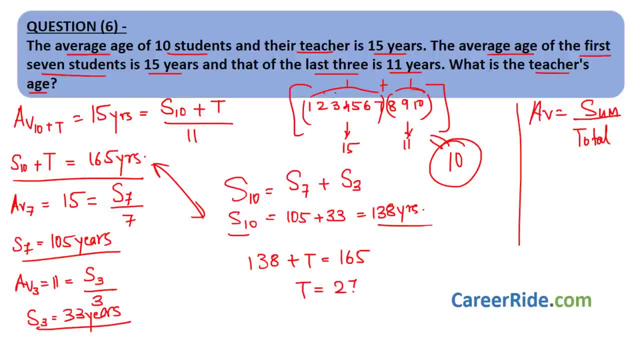 age of teacher is 165 minus 138, 27 years. So this is 168 plus 168.. So this is 168 plus 138.. So this is the age of the teacher. See how easily, using this small formula, we can calculate any sum related to average, Okay, And especially average age. Moving to next, 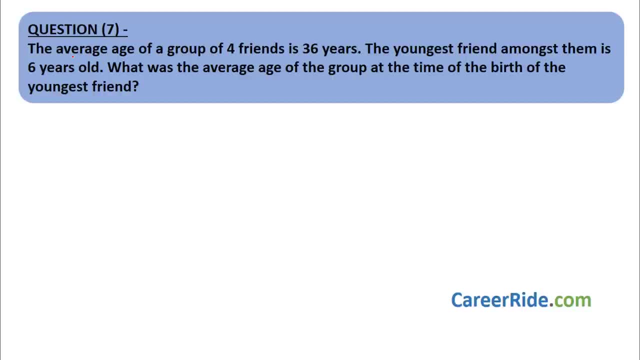 question, Question number 7.. The average age of a group of 4 friends is 36 years. The youngest friend amongst them is 6 years old. What was the average age of the group at the time of the birth of the youngest friend, Right? So the average age of the group at the time of the birth of the youngest friend Right. So the average age of the group at the time of the youngest friend. So the average age of the group at the time of the youngest friend. Again, this is an average sum. so we will have the average is equal to sum of all observations. 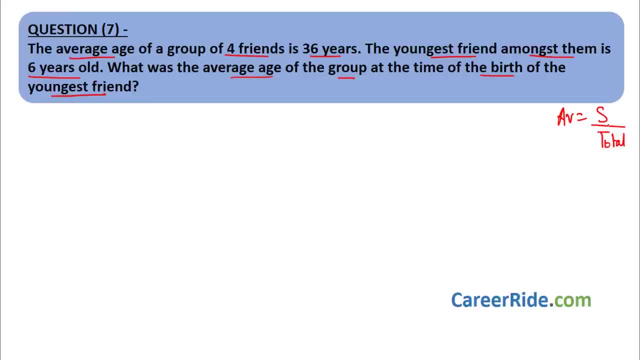 upon total number of observations. That is sum of the ages of all the 4 friends divided by total number of friends. Okay, So the average age of a group having 4 friends- okay- is nothing but 36 years. That is nothing but sum of the ages of 4 friends divided by total number. 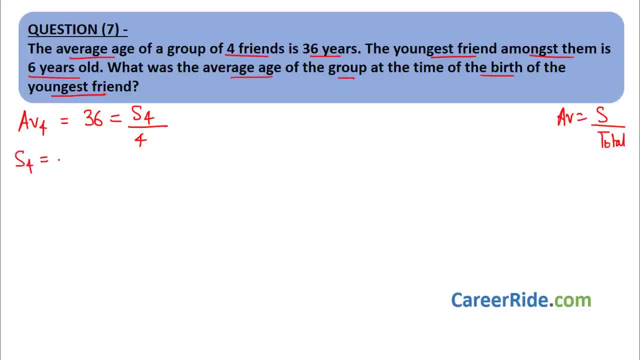 of friends that is 4.. So sum of the ages of 4 friends, 36 into 4, is 144 years. Right Now, What they have given is that the youngest friend which is there is 6 years old, And we want the average age of the group at the time of the birth of the youngest friend. 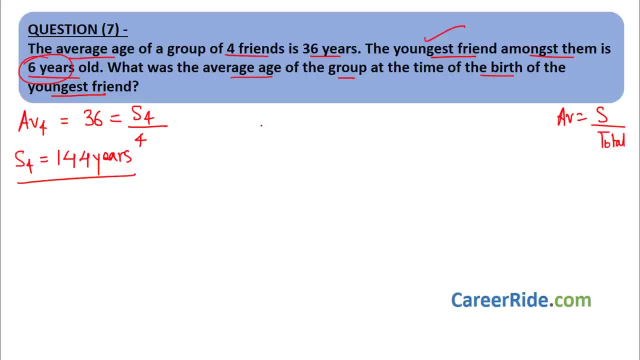 If a person is 6 years old, that means that person must have been born 6 years ago, right? So the youngest friend was born 6 years ago. So when the person was born, when the youngest friend was born, we want the average age of the group. 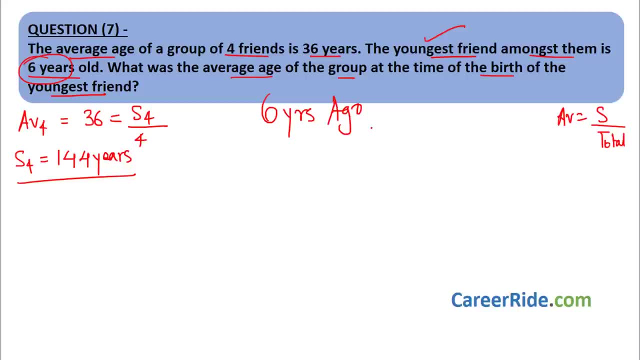 So let's go back 6 years. okay, go back six years. go back six years. now, when we go back six years, what happens is that every friend's age will reduce by six years, correct? so the first friend's age will reduce by six years, seconds would be reduced, thirds also reduce and the fourths also would reduce by six years. 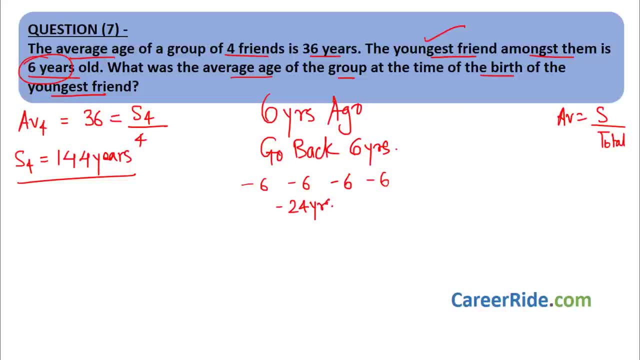 so total reduction would be minus 24 years, right when we add this. so whenever we add the ages of the friends six years ago, the total reduction in the ages would be 24 years. so some of the ages of four friends- how many? six years ago would be 144 minus 24, equal to 120 years. 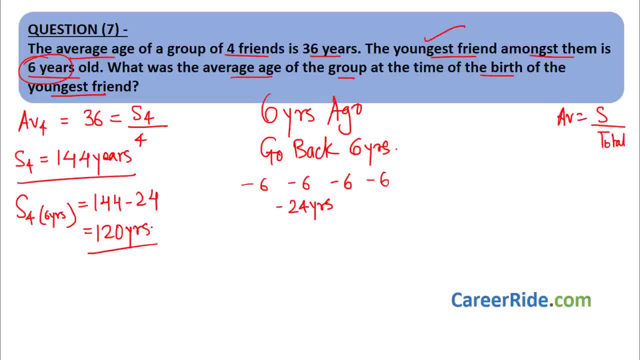 correct now, at this point, okay, at this point, total number of friends are four, but we know that one of the friend which is there- the youngest friend- okay, the youngest friend- he was just born. six years ago. that youngest friend was just born. that means his age was zero years, so is there any need to include his age. 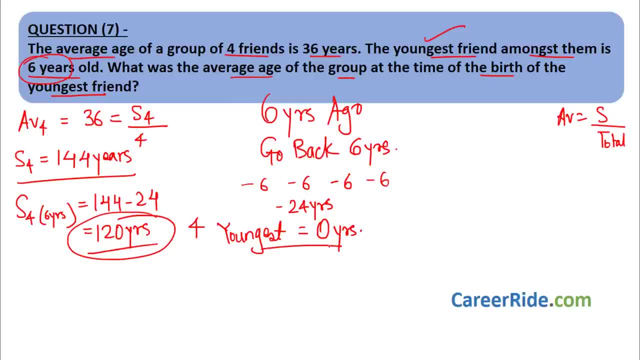 no, so there is no need to include his or her age into this. so total number of friends are not four. but total number of friends are four minus one, equal to three. okay, right, so again, average of the group six years ago. what will have some of the ages of friends? 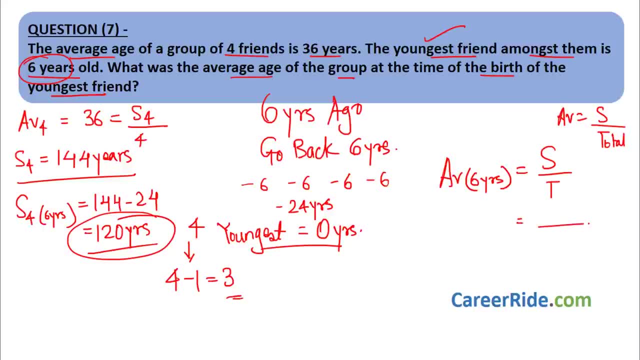 divided by total number of friends, we know the total number of friends as three. why? because the youngest, youngest one was just one and his or her age was zero years. so we need not consider the youngest person, we only consider the other three friends, correct? so total number of friends are three. what is the 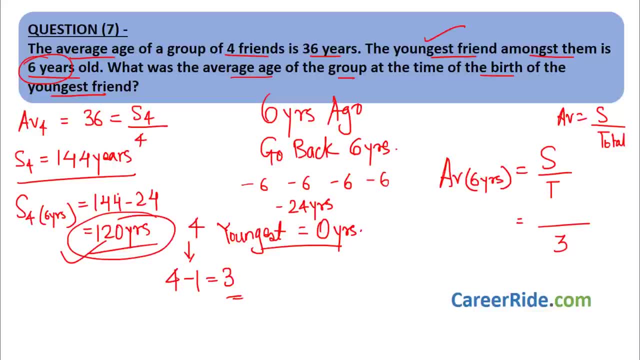 summation of their ages: 120 years. initially it was 144. then we reduce 66 years for each friend so we'll get 120 years right. so that is nothing but 40 years. so average age for the group six years ago- how much six years ago, when the youngest friend was born- is 40 years. see how easy it was. 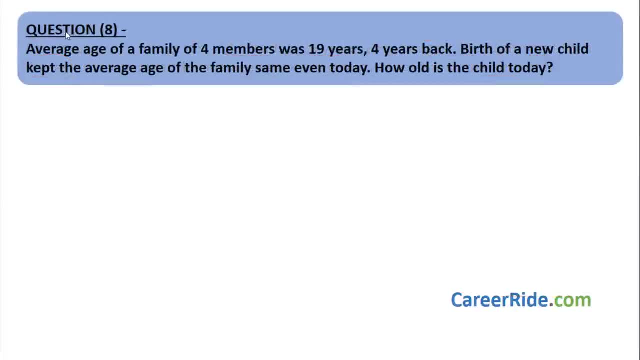 moving to question number eight. question number eight: average age of a family of four members was 19 years. four years back, birth of a new child kept the average age of the family same even today. how old is the child today? again, we have the average sum. so we'll have average as sum of observations divided by total number of. 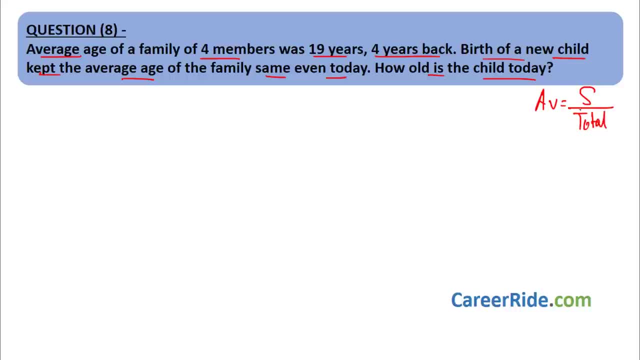 observations. so here it would be sum of the ages of all family members divided by total number of total number of family members. now they have given that the average age of the family of four members was 19 years when it was four years back. so if this is the present age, 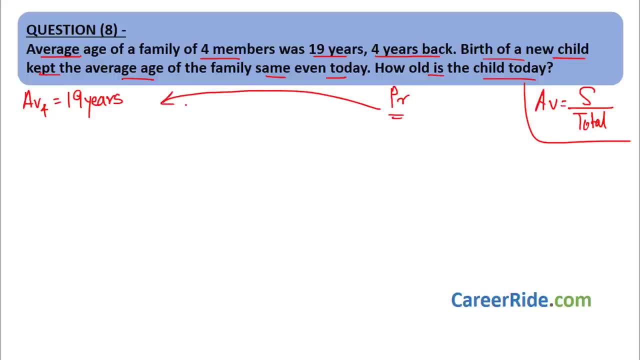 okay, this is the present times, then let us move four years back. okay, so we have moved four years ago. four years back over here, average age of the family members was 19 years. do you know what is average? average average is nothing but some of the ages of all the four family. 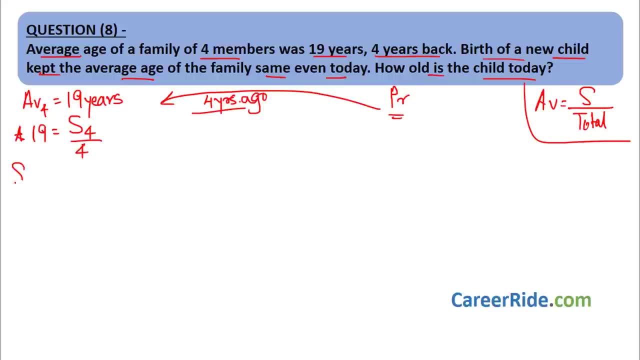 members divided by total number of family members, that is nothing but four. so some of the ages of four family members is 19 into 4 as 76 years right now. the previous sum: we saw that whenever we have gotten going six years back, every person's age reduces by six years, right. so if we are going four years, 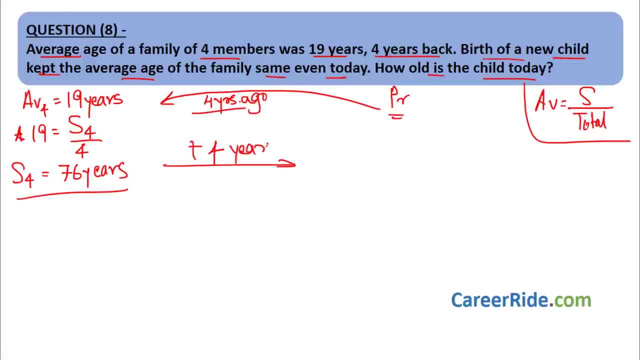 ahead into the future to the present times. okay, so every family members age must increase by four years. so first ones would increase by four, second also four, third also four and fourth also four. all the four family members age will increase by four years. so total increase will be 16 years. 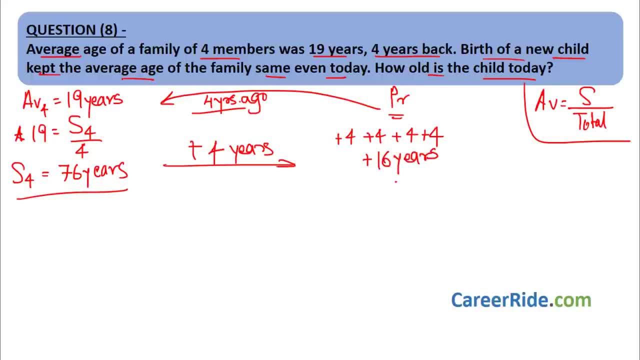 so what would be the present sum of ages of all the family members? very easy, it would be 76 years, that is, four years back plus the increase of 16 years. total increase of 16 years. how much? it is? 70- 92 years, right, 76 plus 16- 92 years. this is the previous four years back addition and 16 years. 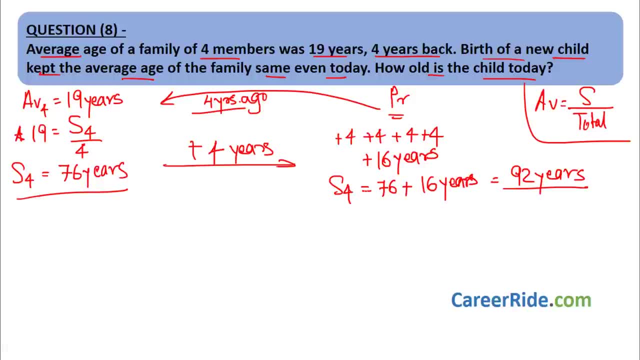 increase four years for each person, so we get 92 years. now this we know. okay. now, somewhere over here a new child was born. do we know the present age of the child? no, do we know when was the child born? no, let us assume that the present age of the child be k years. okay, how much k years now? what is the? 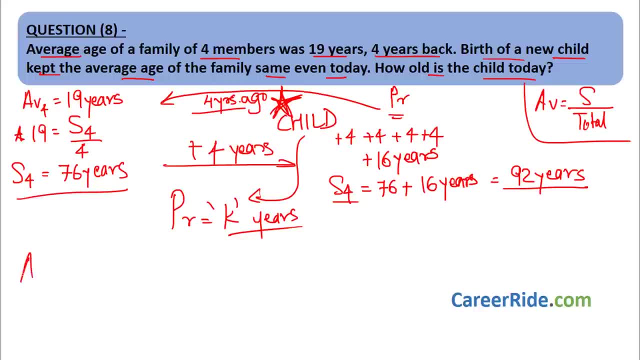 formula for average present average of the family average is sum of the ages of all family members upon total number of family members. total number of family members are four family members plus the new child. that is, four plus one, that is five. sum of the ages of the four family members plus the age of the child. this is the 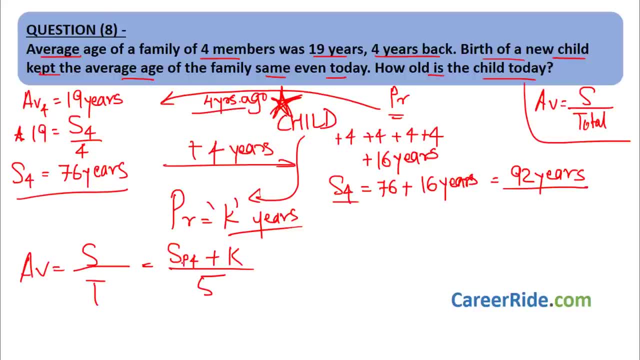 summation. now, what is this? sp4? that means sum of the ages of four family members presently. some of the present ages of the four family members. okay, this is nothing. but this sp4 is nothing but 92 years right presently. so it would be 92 plus k upon five. now here they are, given that. 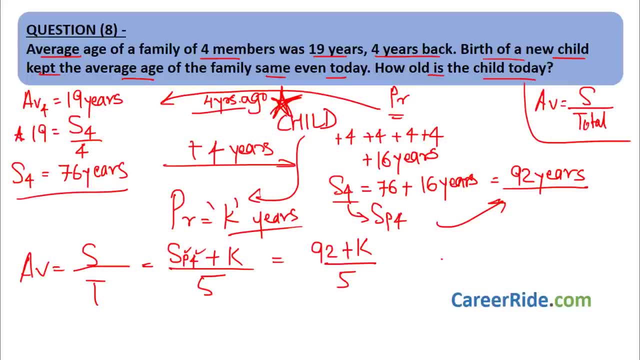 the child kept the average age of the family same even today. so this is nothing but the same. average is same: 19 years. let's see what do we get. 92 plus k would be 19, fives are 95, so k would be 95 minus.